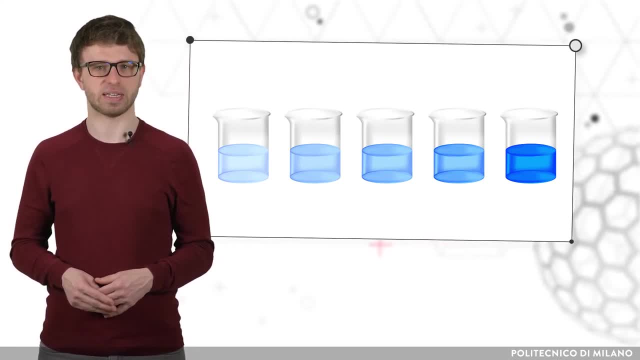 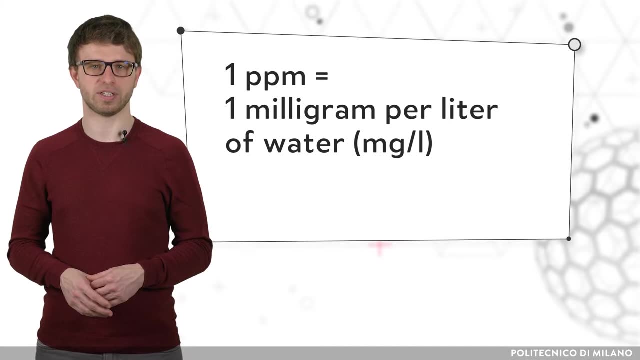 In other words, it can be also described as the number of parts per million. Ppm is also understood as the concentration of a studied element in water or soil When ppm is equivalent to one milligram per liter of water or one milligram per kilogram of soil. 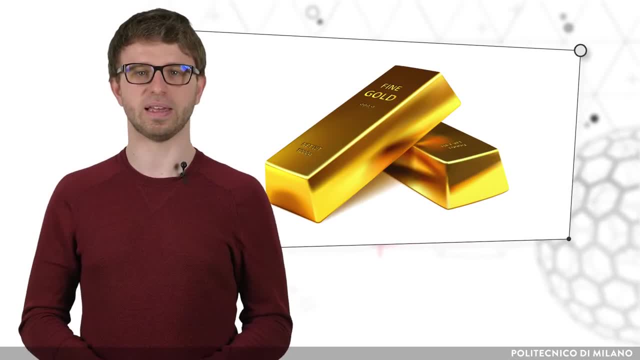 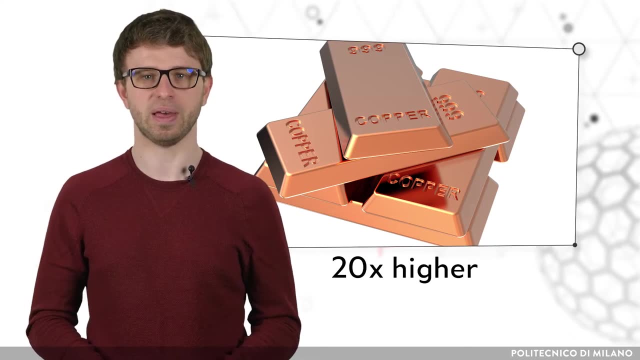 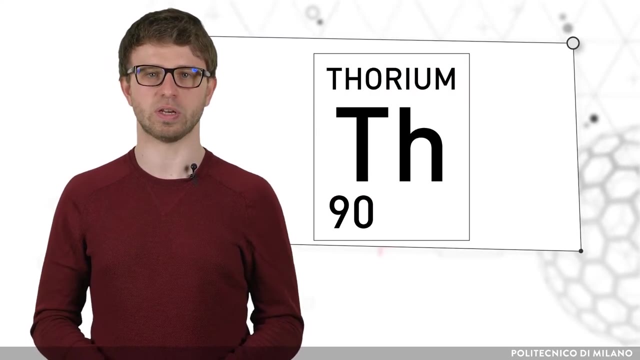 Consider that the abundance of gold is approximately 700 times lower than uranium, while that of copper is around 60 ppm. it means 20 times higher than uranium. An abundance of thorium, which can also be used in fuel in nuclear reactors, is about 10 ppm. 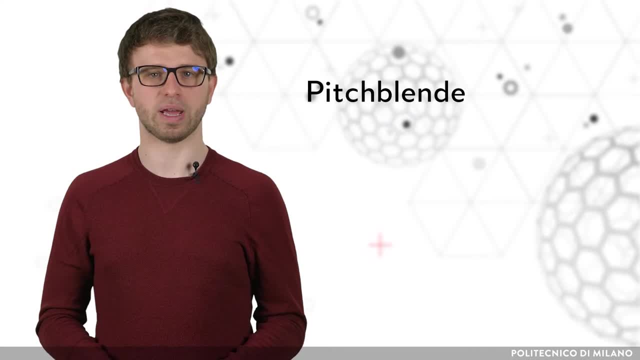 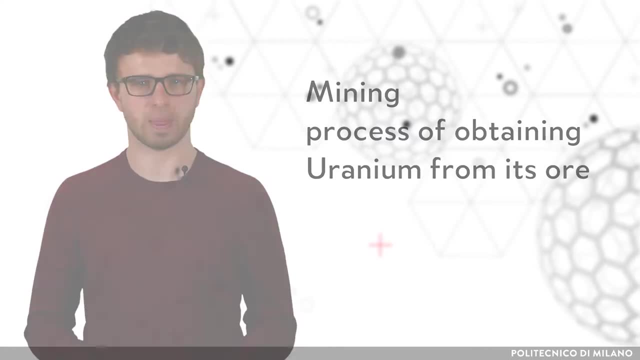 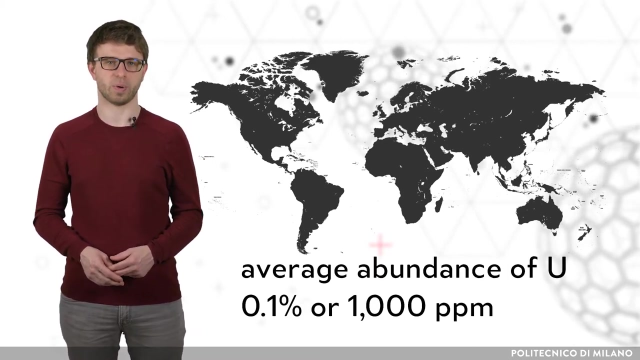 The name of the best-known uranium ore is pitchblende. Miling of uranium is a process of obtaining uranium from its ore- uranium from its ore. In the richest world's mines, the average abundance of uranium is 0.1% or 1,000 ppm. 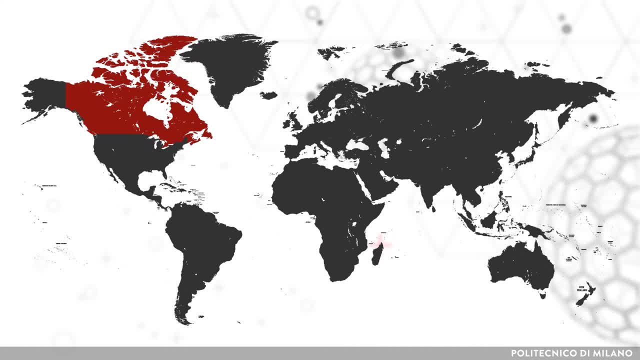 However, in Canada, some mines have vast amounts of ore that have an average grade of up to 20% uranium. Based on this, Canada is the second largest producer of uranium after Kazakhstan. Besides Kazakhstan and Canada, the leading producers of uranium are Australia, Russia. 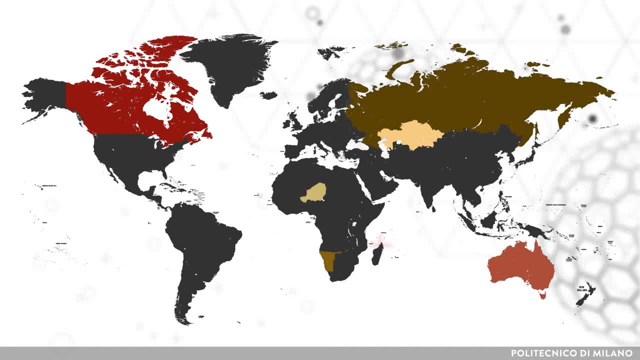 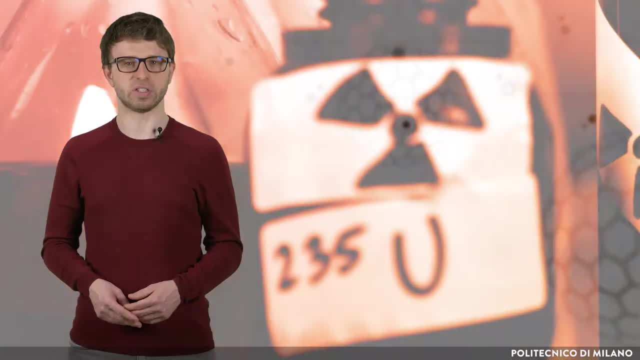 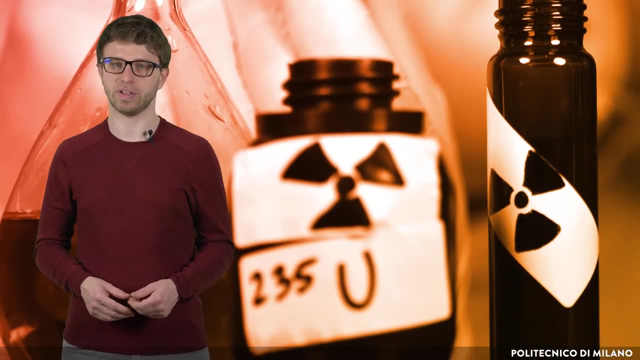 Niger and Namibia. The rest of the countries that operate uranium mines cover approximately 15% of worldwide production. In general, uranium mining is relatively similar to other kinds of mining But because of the radioactivity of uranium ore, special mining techniques are used to. 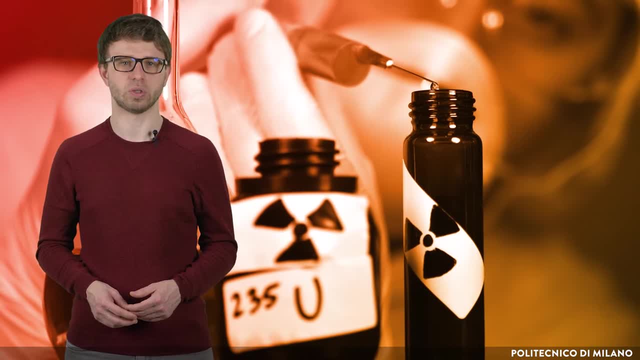 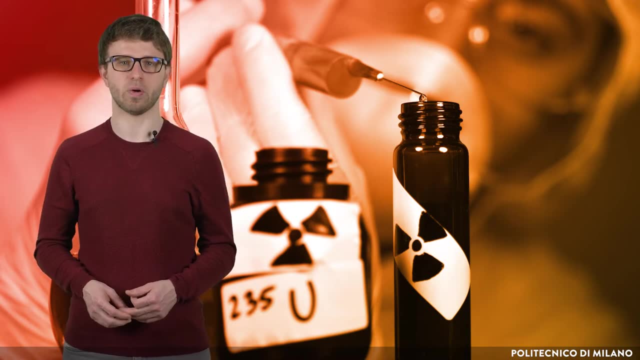 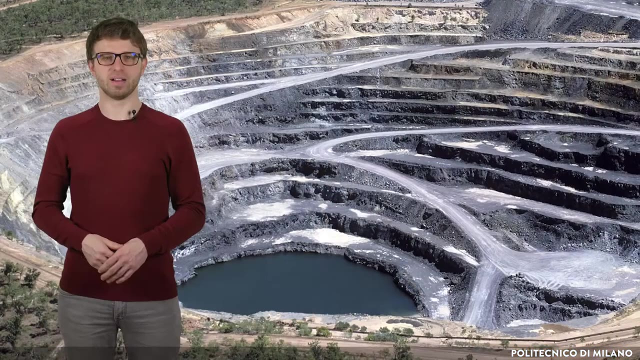 limit worker radiation. In addition, uranium mining is used to reduce the risk of radiation exposure and to ensure the safety of the environment. Depending on the deposit, uranium is usually mined in one of three main ways – open pit, underground mining or underground leaching. 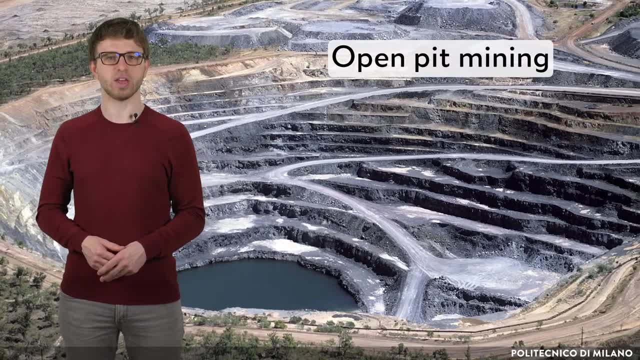 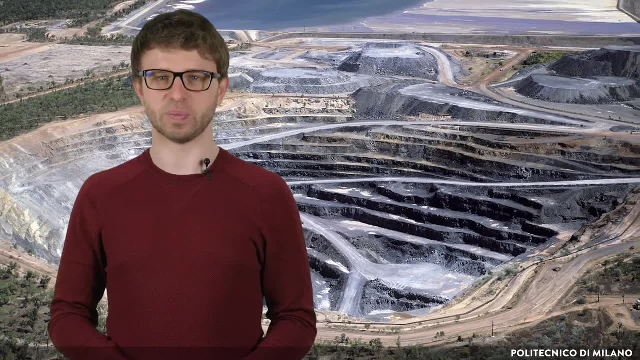 The first possibility is called the open pit mining. This method is used when uranium is found near the surface, usually no more than 100 meters deep. In this method, soil and waste rock is removed by heavy equipment allowing the ore to be accessed. 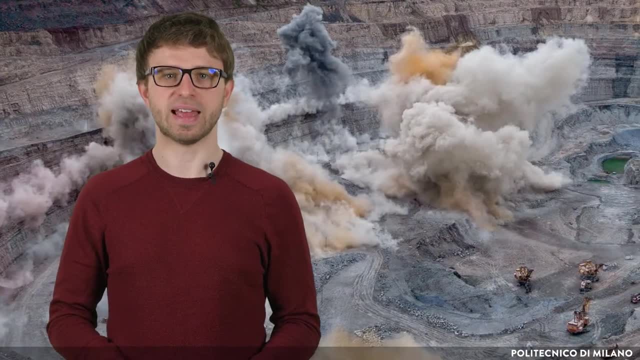 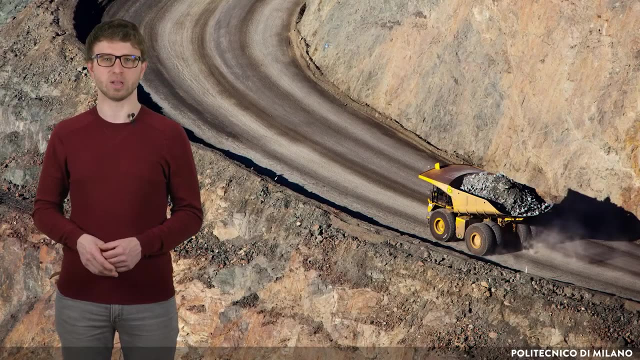 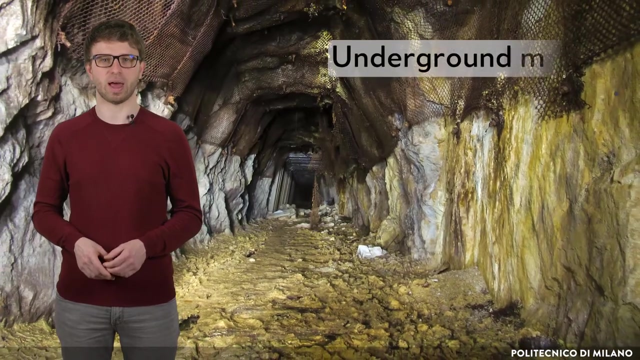 Holes are drilled into the ore and loaded with explosives They detonate, breaking up the rock and exposing the uranium. Once the ore is mined, it is loaded on trucks and shipped to a processing plant. The second way of mining uranium is called underground mining. 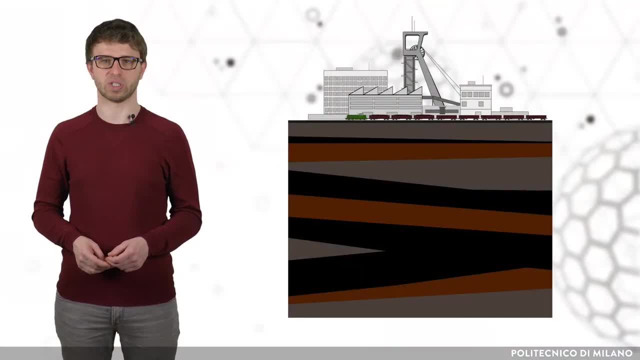 The first step is to dig large vertical underground shafts. This is where uranium is mined, of the ore that can be more than 100 m below the surface. Once this is done, horizontal tunnels, ramps and chambers are built, allowing for the mining. 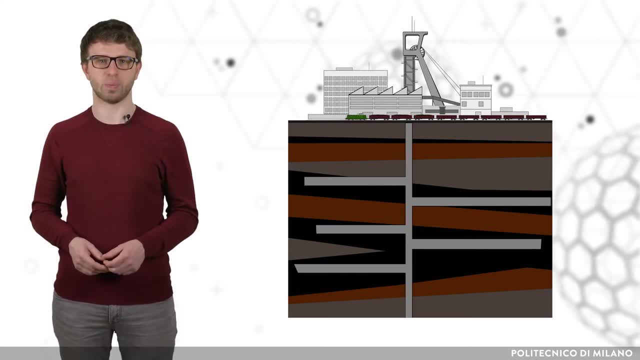 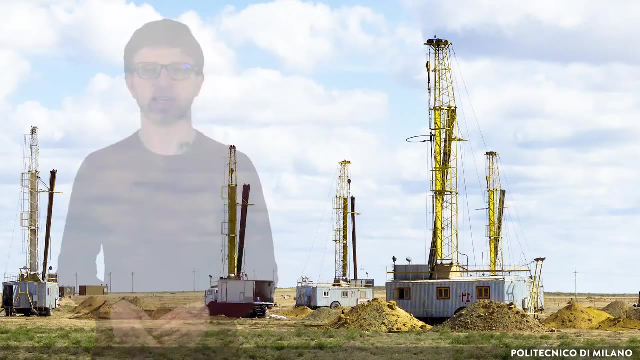 of uranium. There are different techniques to obtain the uranium at this point, but they are mainly based on breaking up of the ore by special dig tools. Mined uranium ore is then moved to the surface and shipped for milling. The last mining method is called underground leaching. 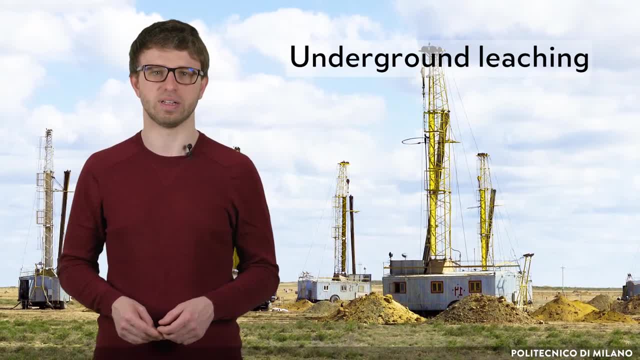 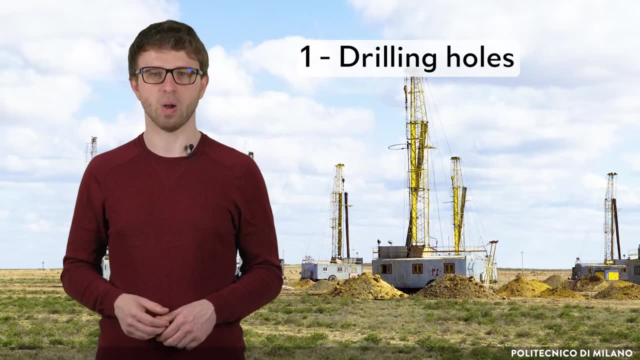 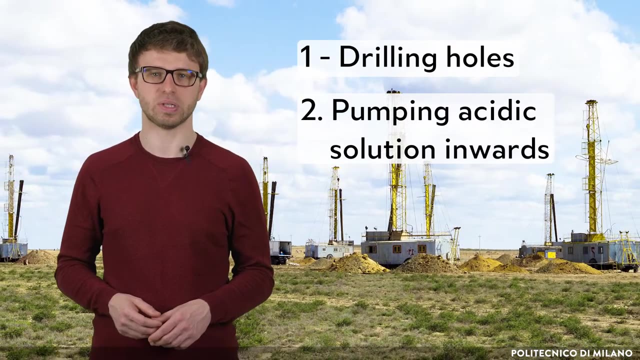 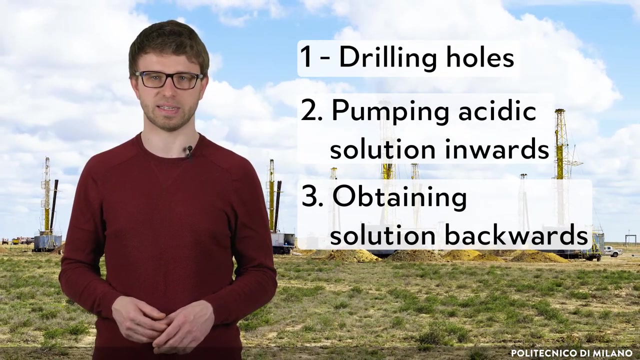 Sometimes geological conditions allow for the dissolution of uranium from its ore directly in the underground deposit. In the first step, holes are drilled into the uranium ore deposit. Next, an acidic solution is pumped into the deposit to dissolve the uranium. Finally, the solution is brought back to the surface and set for further processing to. 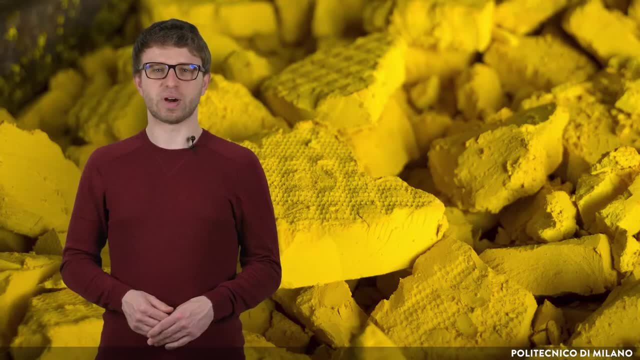 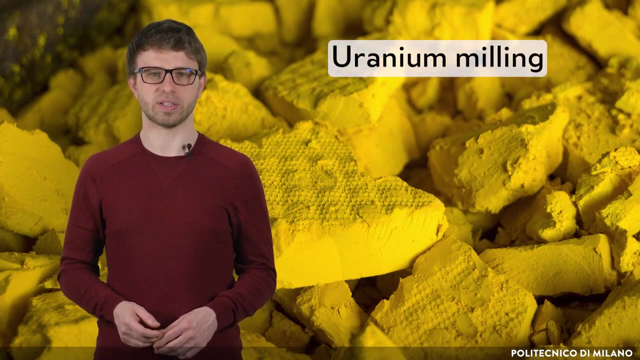 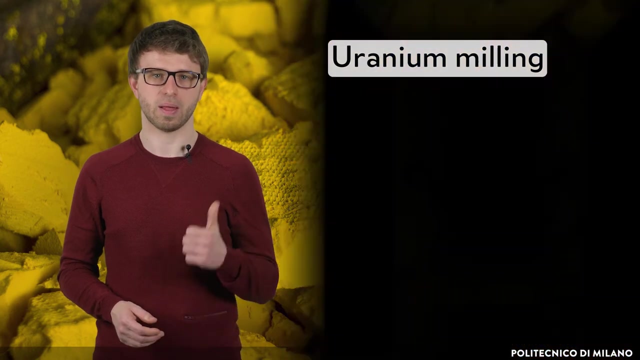 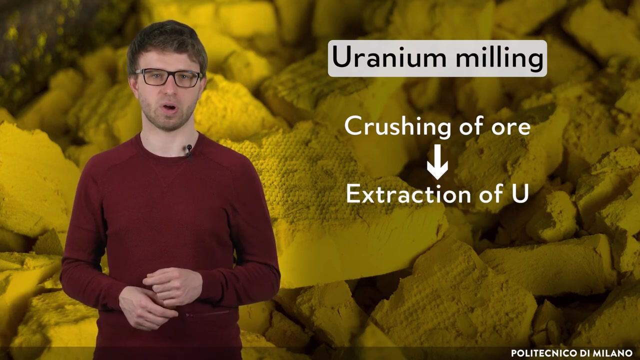 extract the dissolution. After uranium mining, the next step is its milling. that consists of the separation of uranium from its ore. The three main stages that uranium ore undergoes in a mill are the crushing of the ore into small particles, then the extraction of uranium from its ore by using sulfuric acid or alkaline. 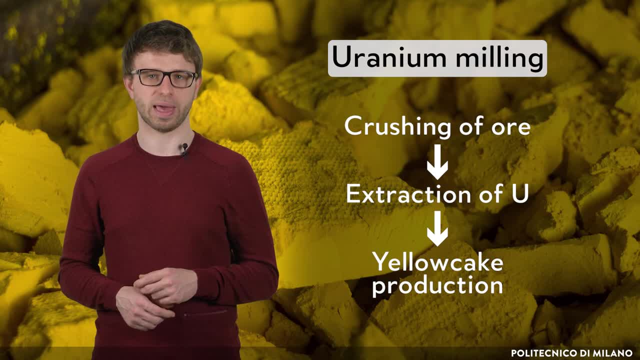 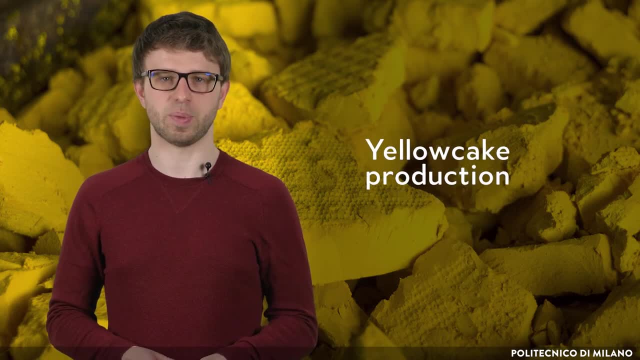 solution, Followed by the production of uranium. The next step is the milling. The next step is the production of yellow cake, which is then dispatched for nuclear fuel fabrication. Yellow cake production is an important step between uranium mining and nuclear fuel fabrication. 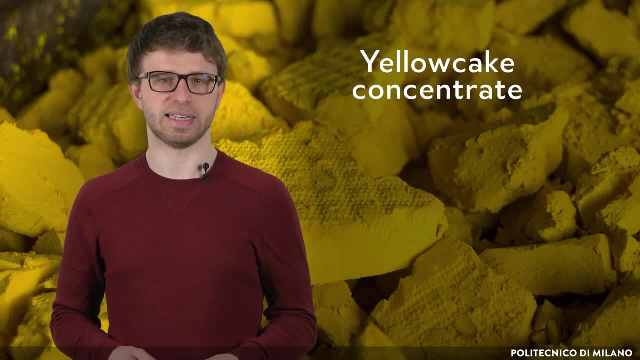 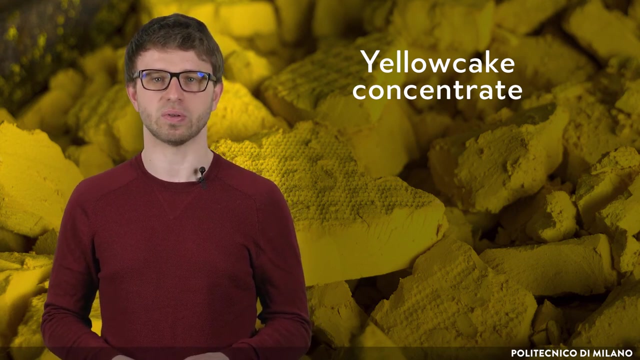 Firstly, a yellow cake concentrate is needed. Its composition can differ and it depends on the type of ore from which the uranium was obtained. It contains uranium in different forms and in different chemical states. Next, the yellow cake concentrate is treated with acid.